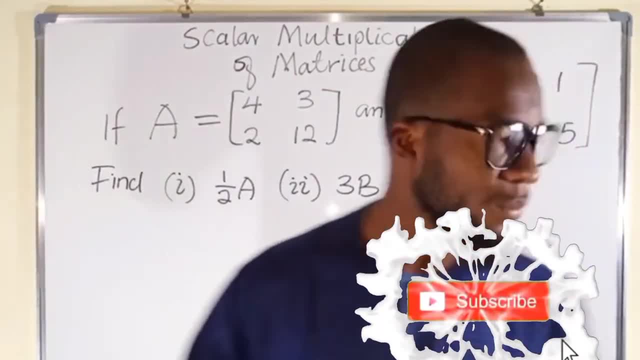 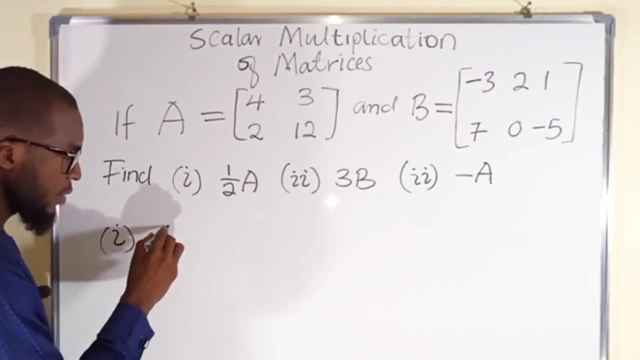 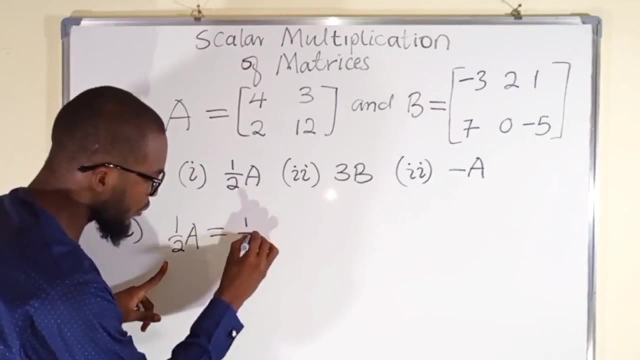 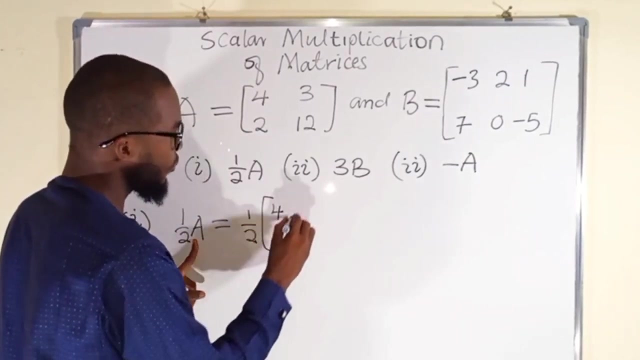 matrix A. So let's begin with this one. What this means We have half of A, half of A is exactly equal to half, which is 1 over 2, then multiply by matrix A, which we have here as 4,, 2,, 3,, 12.. 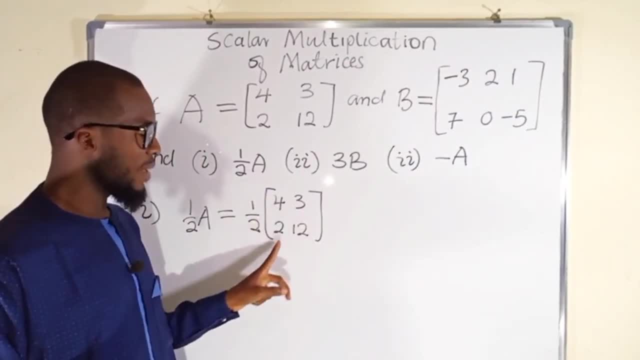 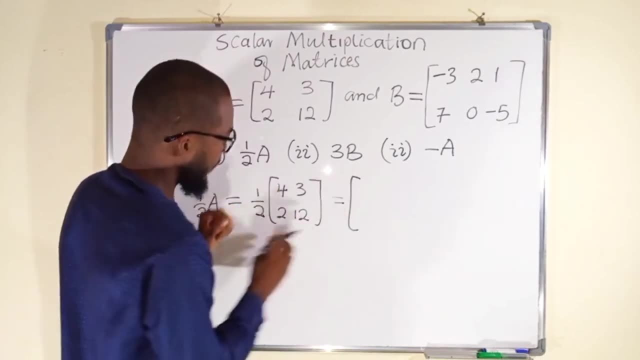 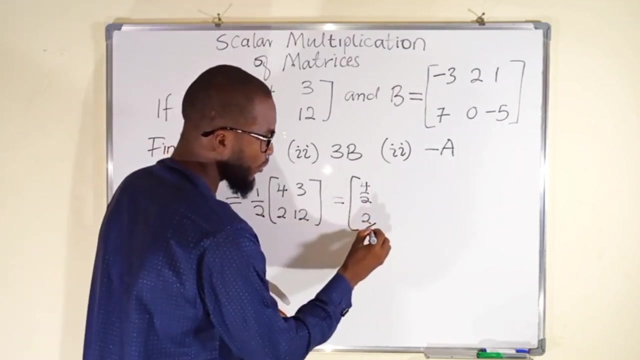 So we are going to use this 1 over 2 to multiply every single element independently in this matrix And this becomes: We have half of 4.. 4 is the same thing as 4 over 2.. Half of 2 is the same thing as 2 over 2.. 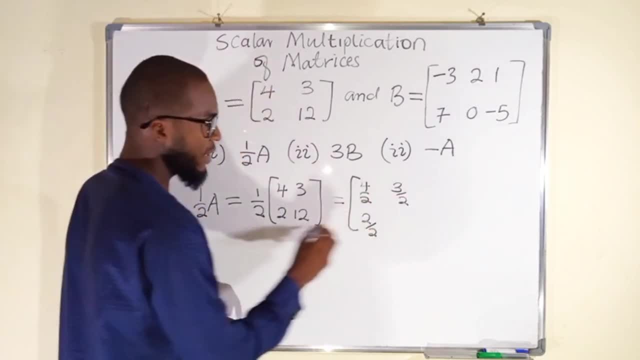 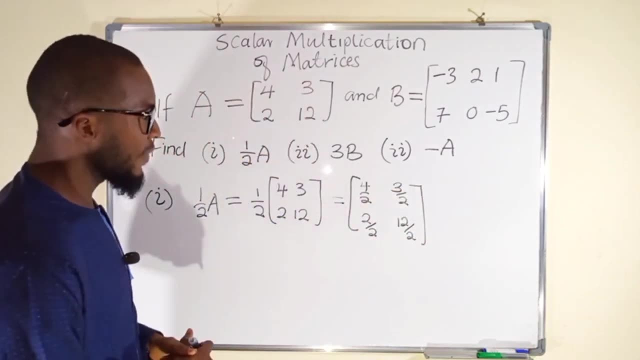 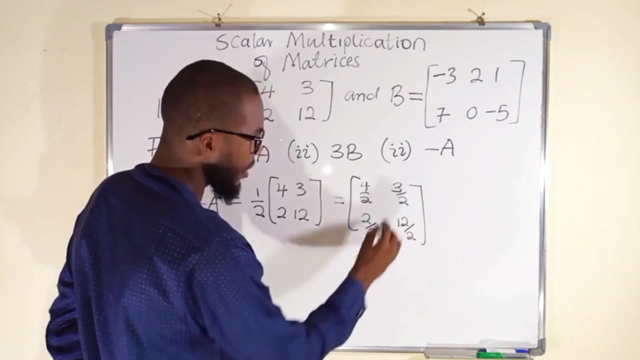 Half of 3 is the same thing as 3 over 2.. And finally, half of 12,, which is the same thing as 12 over 2.. We simplify and obtain our final answer. So this is equal to half of our 4 is 2,. we have 2 here. 3 remain 3 over 2, because we 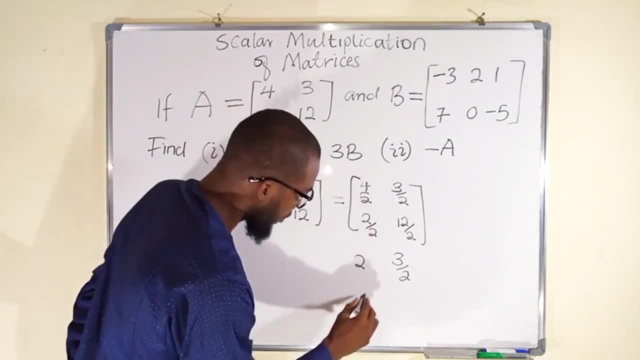 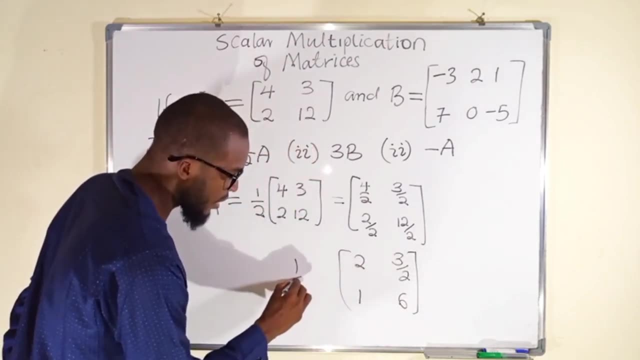 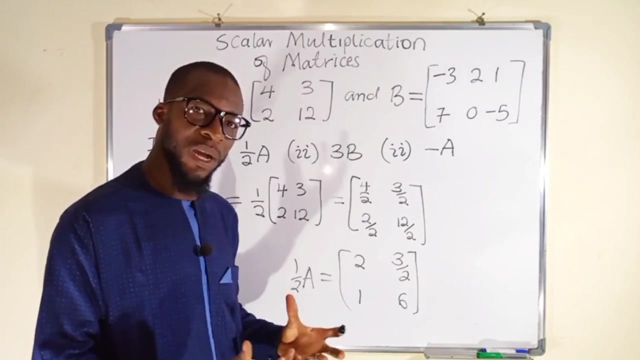 can only simplify it to decimal numbers. This is 1 and this is 6.. So, finally, this is what we have as half of A. It is nothing but just the product of a real number and that matrix. Let us move on to the second one, which is 3B. 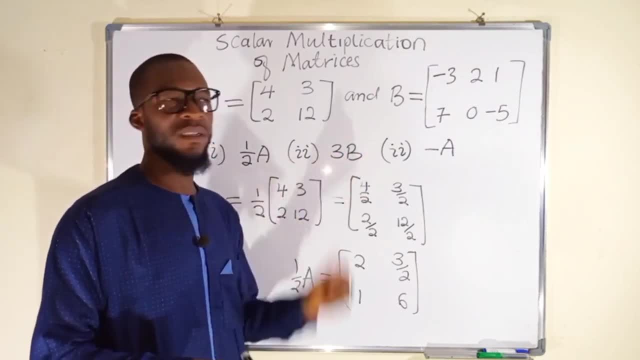 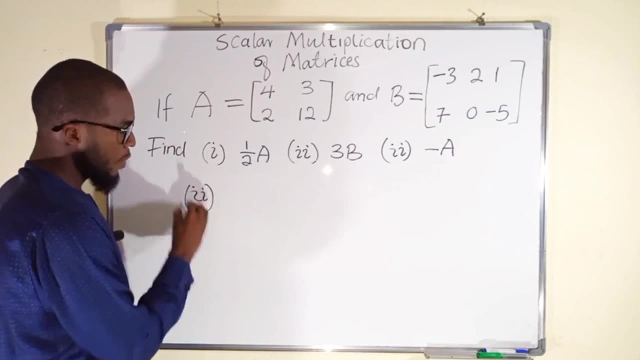 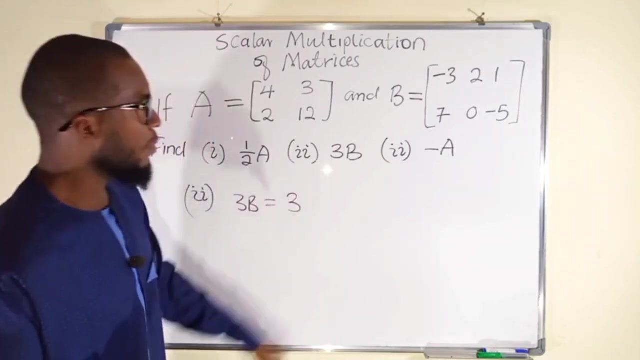 We are going to use this real number 3 to multiply every entry in this matrix B, So Roman 2, we have 3B. and what does this 3B mean? It means 3 multiplied by the whole of these entries. 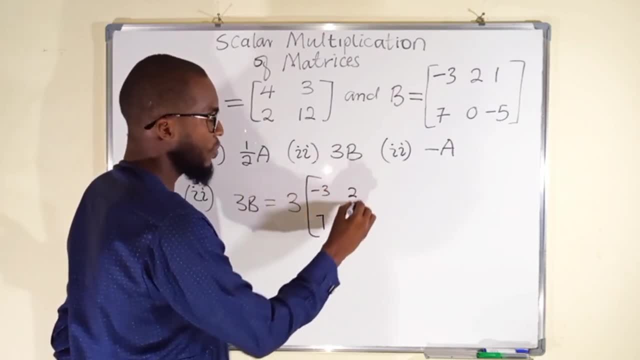 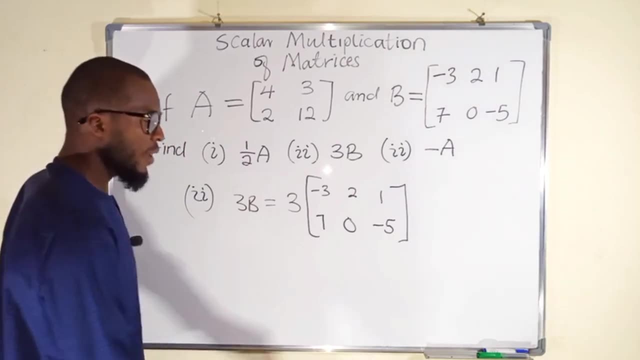 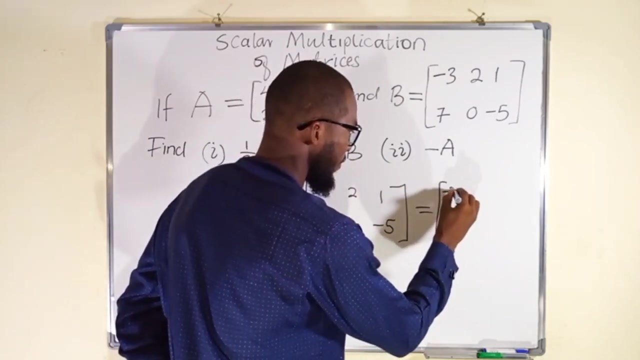 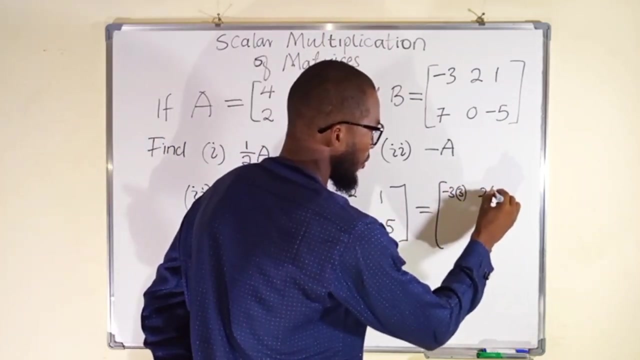 We have negative 3,, we have 7,, we have 2, we have 0,, 1, negative 5.. Alright, this becomes 3 multiplied by negative 3.. So we have negative 3 multiplied by 3,, we have 2 multiplied by 3, and finally, we have: 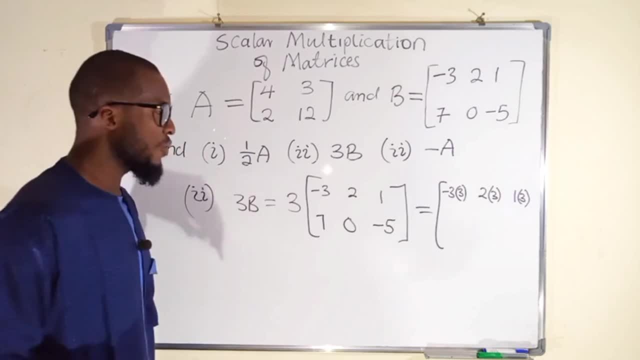 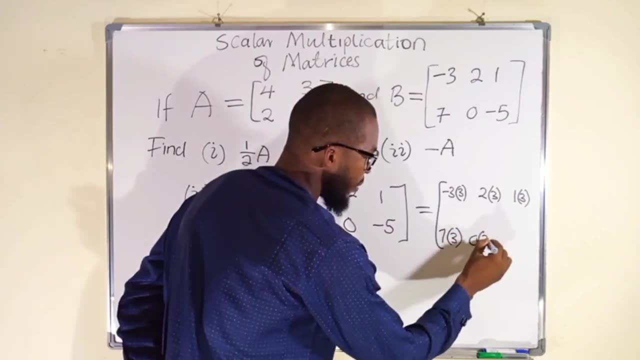 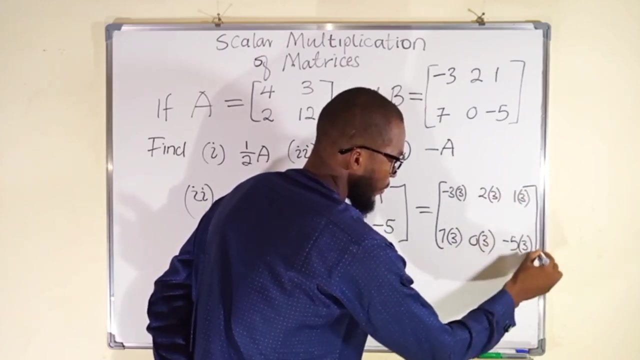 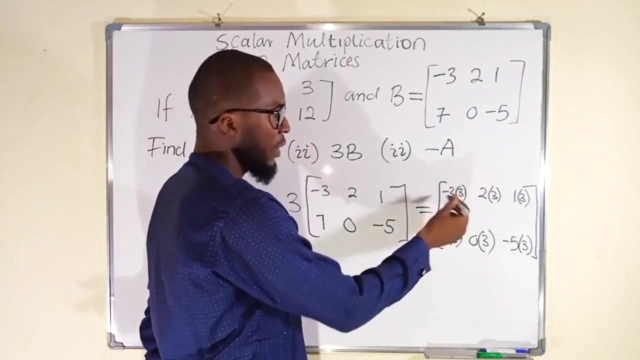 1 multiplied by 3.. In the second row, we have 7 multiplied by 3, we have 0 multiplied by 3, and finally, negative 5 multiplied by 3.. Now let us simplify every entry here: Negative 3 multiplied by 3 is negative 9, so we have negative 9.. 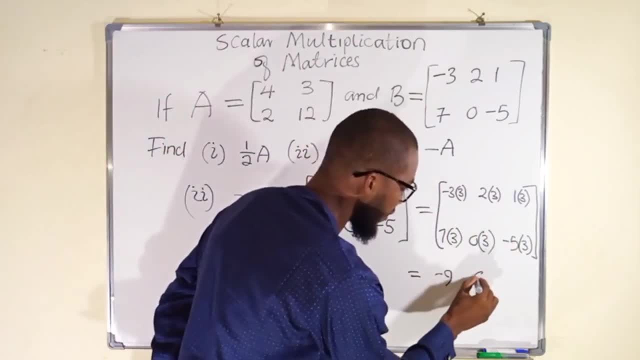 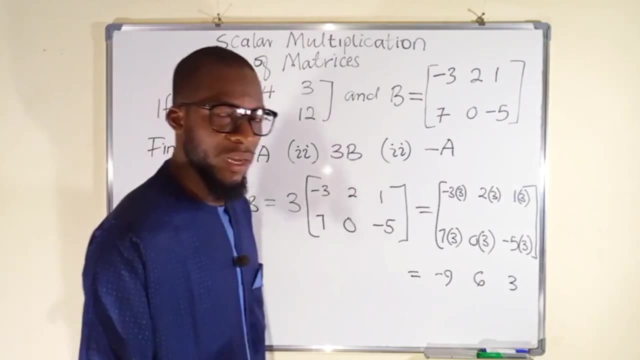 Row 1, column 1, we have 2 multiplied by 3 is 6, so we have 6 here. We have 1 multiplied by 3 is the same thing as 3.. In the second row, we have 7 multiplied by 3, which is 21,. so we have 21 here. 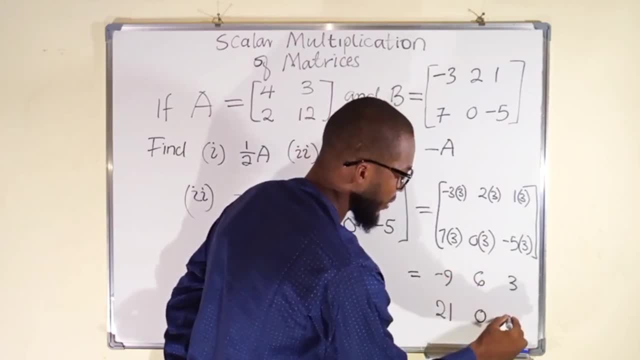 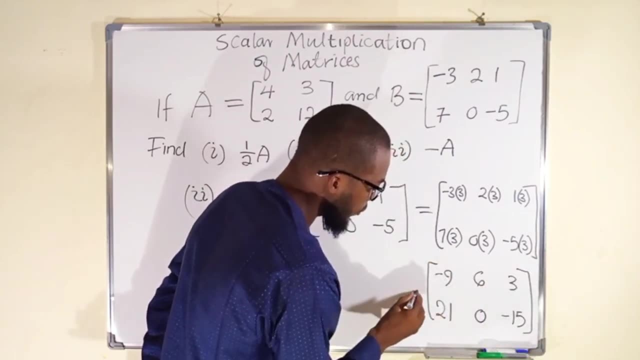 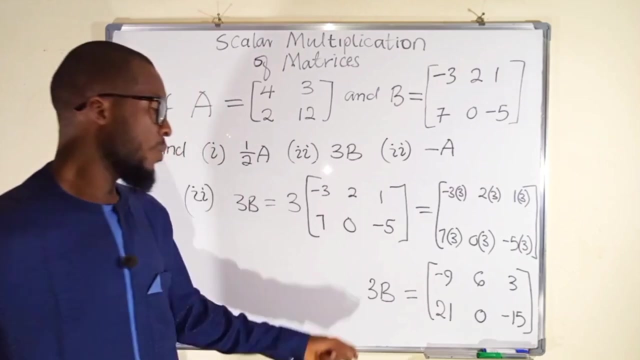 0 multiplied by 3 is 0.. The negative 3 multiplied by 3 is 0. So we have 21 here, And negative 5 multiplied by 3 is negative 15.. So this is equal to 3B. 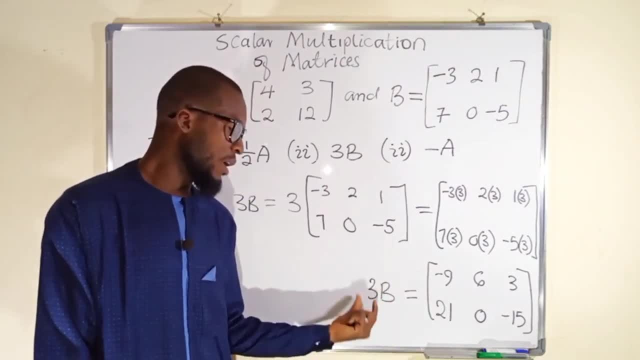 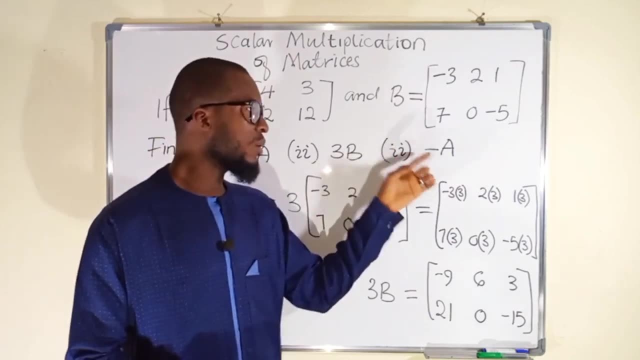 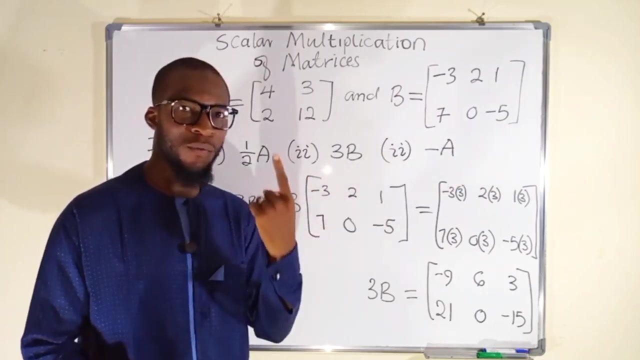 Once you multiply the entries of matrix B by a real number, 3, you will obtain this new matrix. So now let us take the last one, which is negative A. Negative A is the same thing as B, same thing as multiplying the matrix E by negative 1.. So the last one, which is 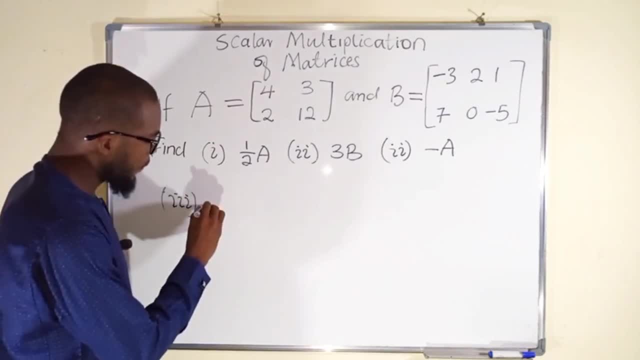 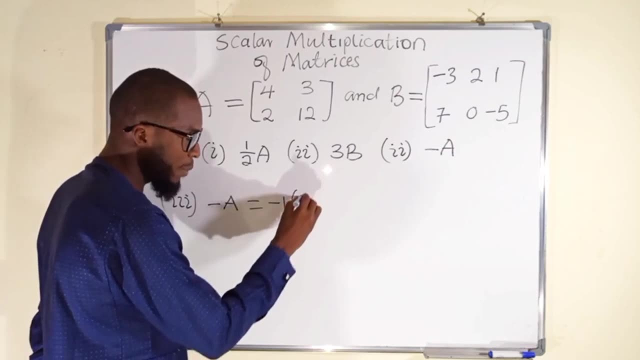 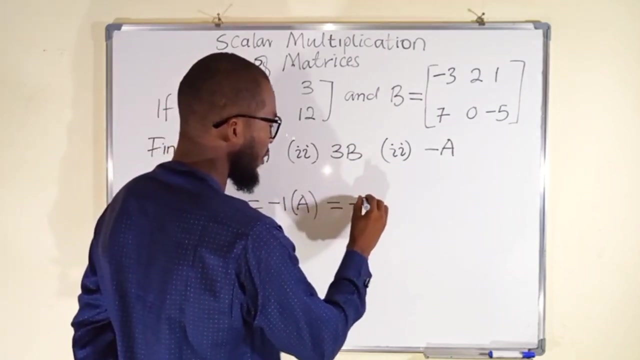 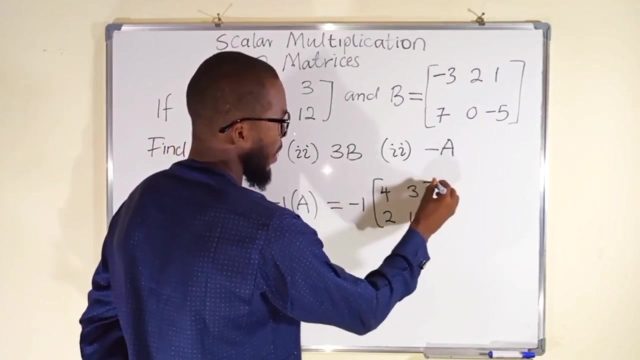 Roman 3. we have negative E, and negative E is the same thing as negative 1 multiplied by E and A is this matrix, so it just becomes negative 1 multiplied by this. entries: we have 4, 2, 3 and 12, so every single element in this matrix will. 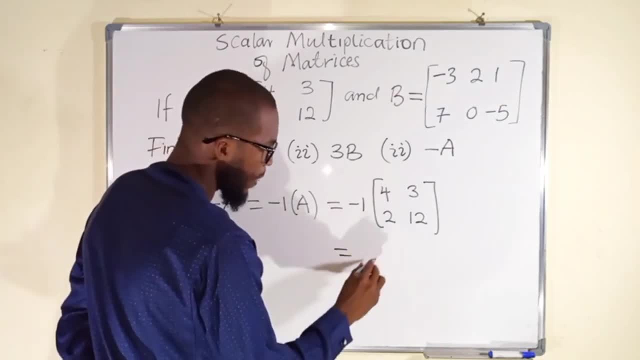 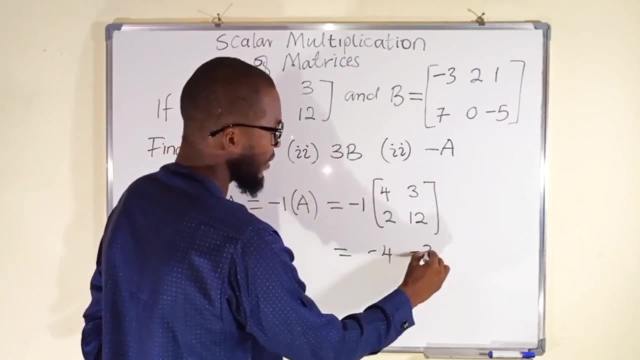 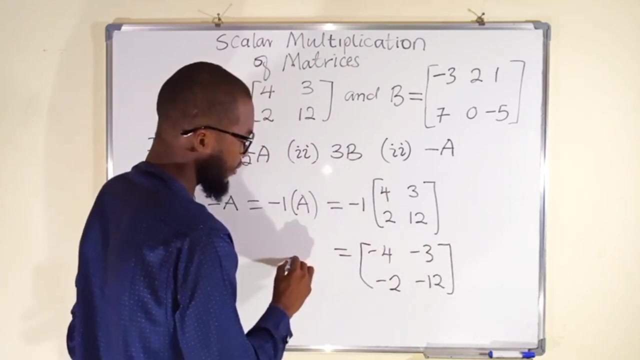 be affected by this: negative 1. so we have- I can just read directly: negative 1 times 4 is negative 4. negative 1 times 3 is negative 3, negative 2, negative 12. so this is our new matrix, which is negative E. 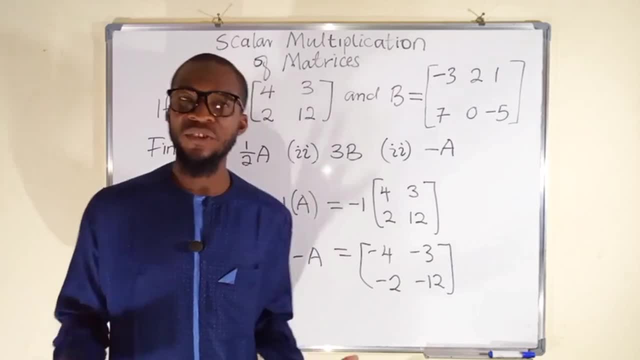 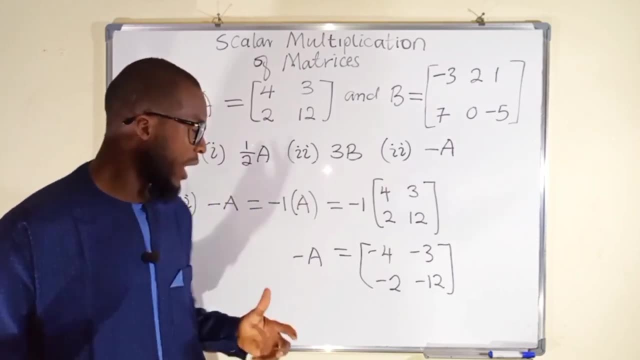 you. so scalar multiplication of matrix is nothing but just the product of that alien number and the given matrix, and this is all I have for you today. thank you for watching. do have a nice day.